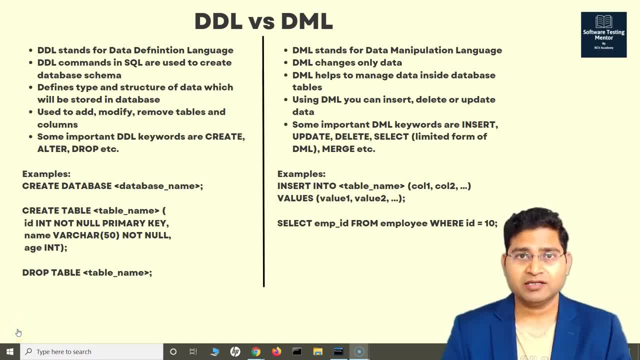 Hey everyone, welcome back in this SQL tutorial. We are again going to understand one of the very important interview questions: What is the difference between DDL and DML in SQL? So DDL stands for Data Definition Language and DML stands for Data Manipulation Language. Now, if you deep, 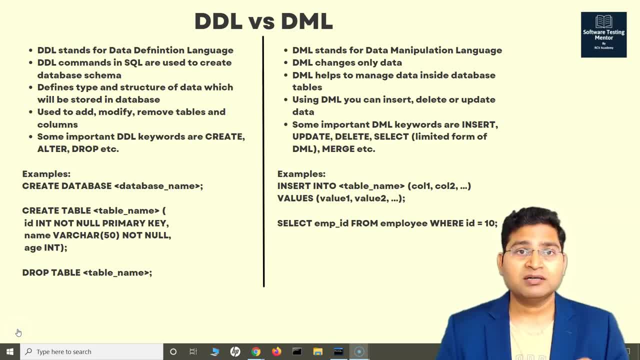 dive into the meaning of definition and manipulation. the answer lies within these keywords itself. So when we say definition, that means we are defining something right. When we say manipulation, we are manipulating something. So, briefly, things are a little bit clearer. So now, 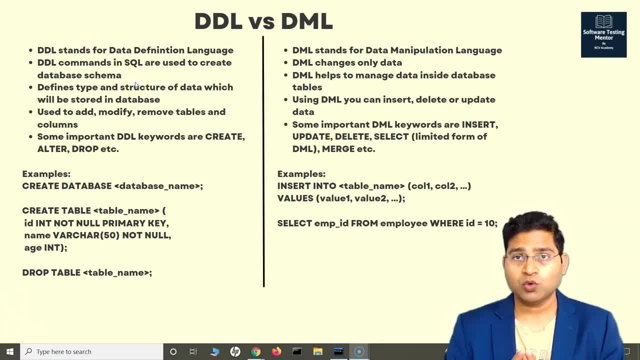 if we go to the details of Data Definition Language, so what it stands for it's basically data definition. It defines something. So DDL, or Data Definition Language, is used in SQL to create a database schema When we say create database schema. so basically it helps you to create the 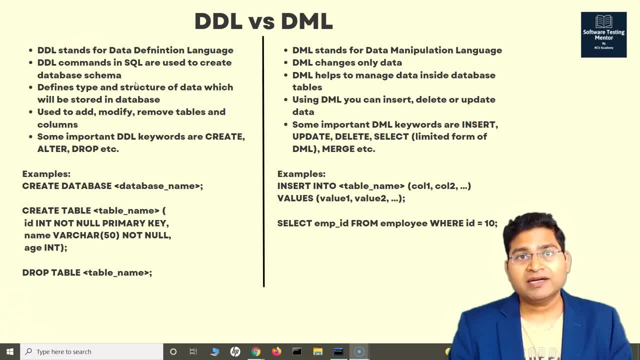 database structure, Then what tables will be there? Which columns will be there in the table? Say, for example, I am creating a database for the company, right? So I create a database with the name company. So that's what I'll do through the data definition language When we create the 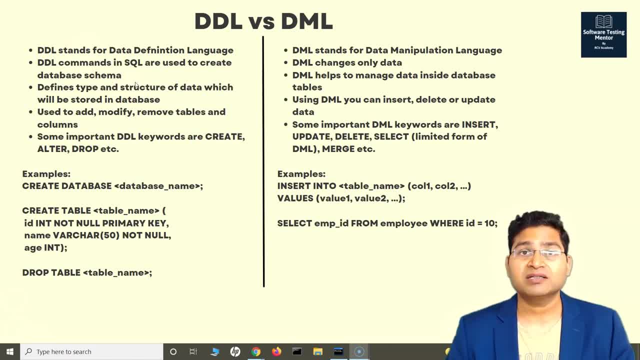 database, then we switch to that database. We then create the tables within the database and within the table we define that these will be the columns. Each column will hold these sort of values. This column- employee ID column- will hold integer name, will hold the characters, etc. So 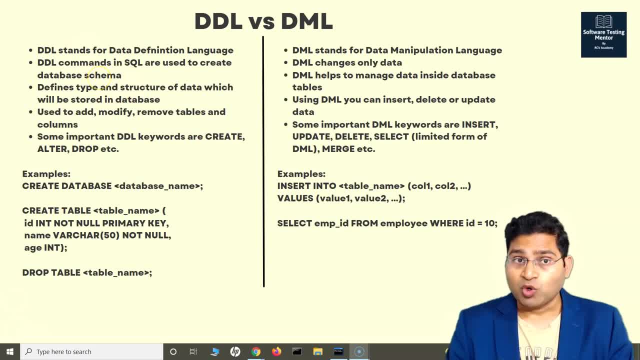 this is being defined by data definition language. Some of the important data definition keywords are create, alter and drop. So data definition language is defining language for the database, the tables, etc. The constraints: everything right. It defines the structure or the schema of. 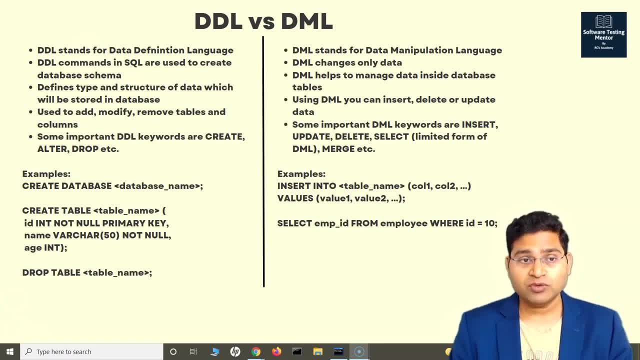 the database. Some of the examples of database or data definition, language, for example, creating database: right. So we create a database, So create database and the database name. So this is more of a defining. We are defining the database right. Then we are creating the table, So create table. 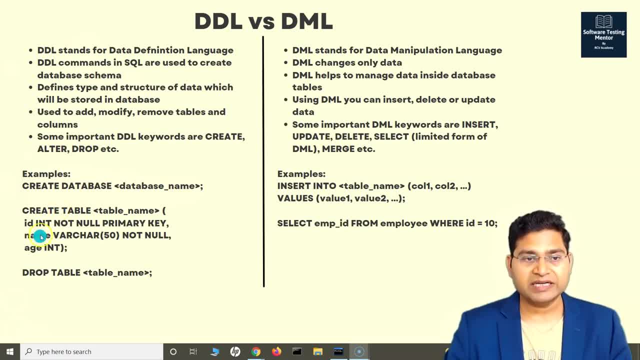 We are creating something, So create table with the ID name. These are the columns. So we are again defining the table within a particular database, or we are dropping the database, or dropping the table. We are deleting it, right. So we are actually defining the schema or we are updating. 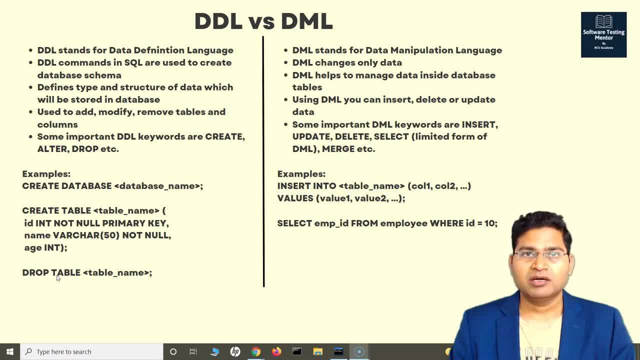 the schema, right. So when we define something, when we ensure that we are defining database, defining table, defining constraints, that's what data definition language is. And then we data definition language is all about and it's a SQL statement, right, but the differentiation is that 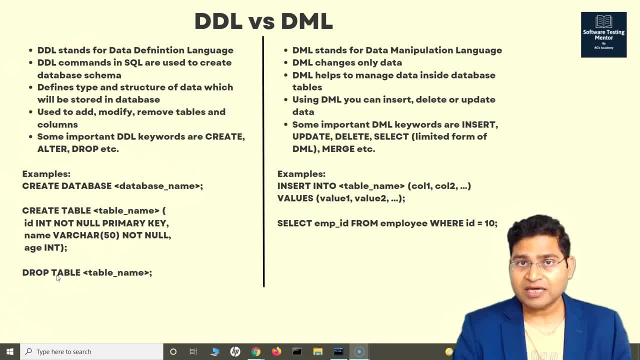 when we define something, we categorize that as data definition language, and when we manipulate the data within the table that is stored, that's data manipulation language, right? so, as the name suggests, data manipulation language. so what it stands for? it stands for data manipulation language, DML. it changes only data, so data that is stored within the table. so, once you have defined database, 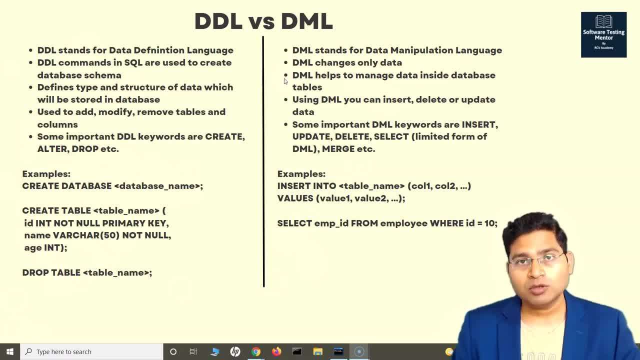 once you have defined how many tables will be there, which columns will be there, the next thing is you will populate the data right. so, for example, employee personal information is the table that you created. now table will be empty initially. then you will be inserting some data data there. 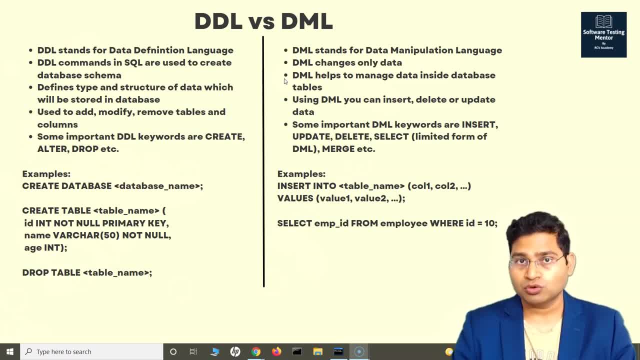 right. so you insert the data within those table. so what you are doing- you are manipulating the data, right? you are actually working with data and trying to push that data within the table that you have defined. so that's what data manipulation language is all about: when you try to push the data within the table, try to fetch the data, try to update the. 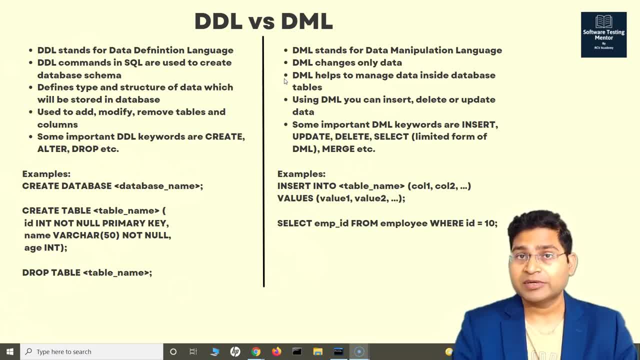 data right. anything that you do with the data within the database and table is done by the data manipulation language and please remember DDL versus DML. the differentiation is the way you use these SQL queries, but both of them are the SQL query right, so they are the queries of the 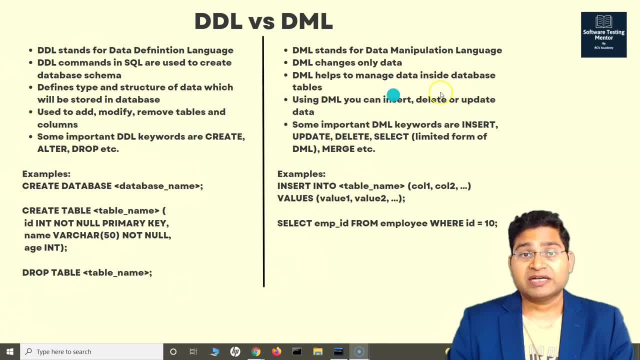 structured query language. so DML helps to manipulate, manage data inside the database table using DML so you can insert, delete, update the data right and some of the important DML keywords are: insert, update. you know, delete, select is limited form of DML because when we say select we are fetching. 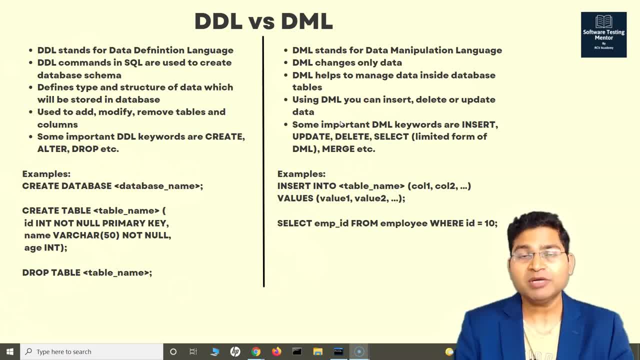 the data, but we are not sort of updating. so it's a limited form of DML, but it is a data manipulation language keyword as well. okay, then there are much, so you can go through Google search for DML statements, go to go to Oraclecom, some genuine sort of website, and you will get all these.